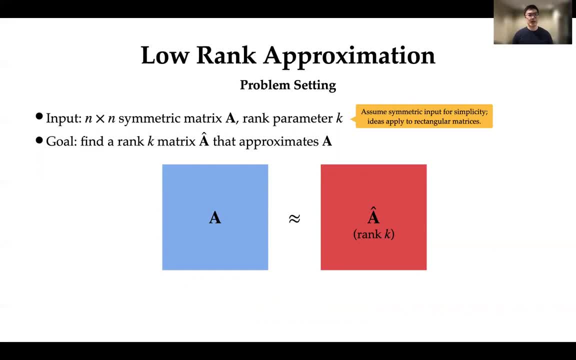 problem. So in this problem we're given as an input an n-by-n symmetric matrix A as well as a rank parameter k, And our goal is to find a rank k matrix A hat that approximates A in some sense, And usually this A hat is found by finding the matrix X that minimizes. 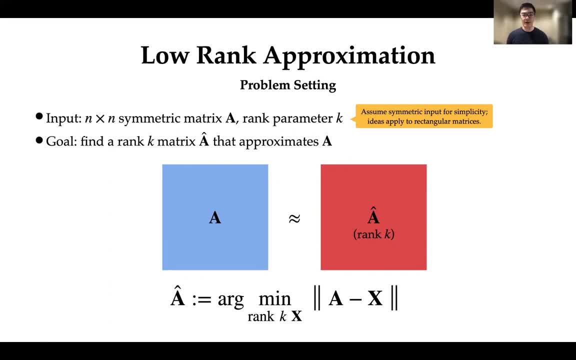 A minus X in some norm over the space of all rank k matrices, X. Here the norm can be chosen to be the Frobenius norm, spectral norm or the entrywise LP norms or a variety of other selections. But for the purposes of this talk we'll be focusing on the spectral norm. 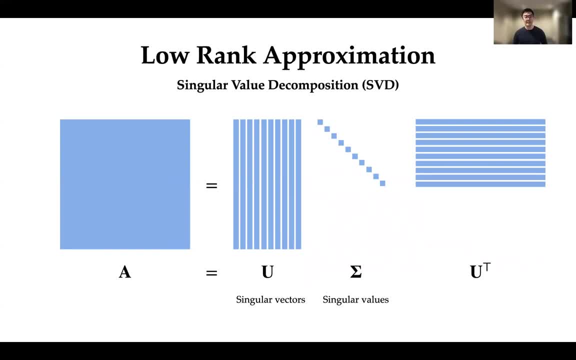 Now, in order to discuss our results, I'll introduce the singular value decomposition, or the SVD. So in the SVD we can take a symmetric matrix A and write it as the product U times sigma times U transpose, where U is a matrix that has orthonormal vectors which are known. 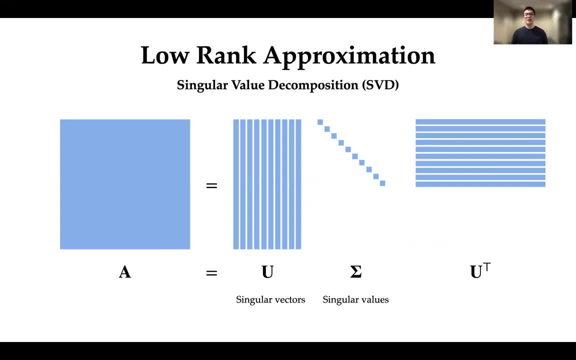 as the singular vectors along its columns And sigma, is a diagonal matrix that has the singular values down its diagonal. Now, associated with the singular vector, we can write: the SVD is a natural matrix, A, k, which is a rank k matrix that can be obtained by taking just. 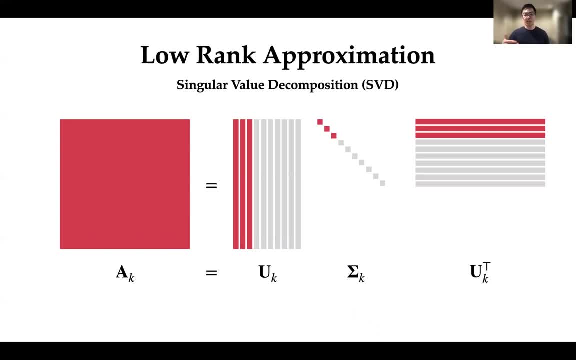 the top k vectors of the singular vectors, as well as the top k singular values, And by the Eckhardt-Young-Mersky theorem. this is known to be optimal for Frobenius, or the spectral norm Lorentz approximation problem. 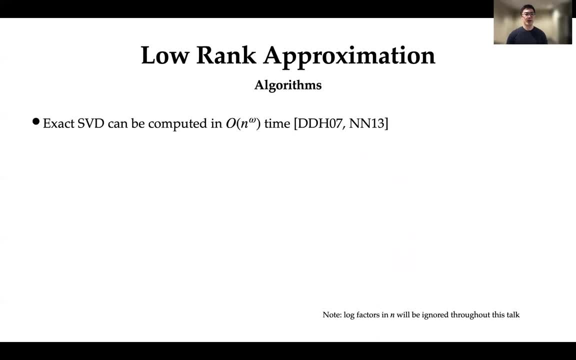 Now, in terms of algorithms, it's known that the exact SVD can be computed in time, N to be omega. So here is the exponent of matrix multiplication. Now, if we're willing to settle for approximations, then it's also known that an approximate SVD can be computed in O of NNZ of A times k over. 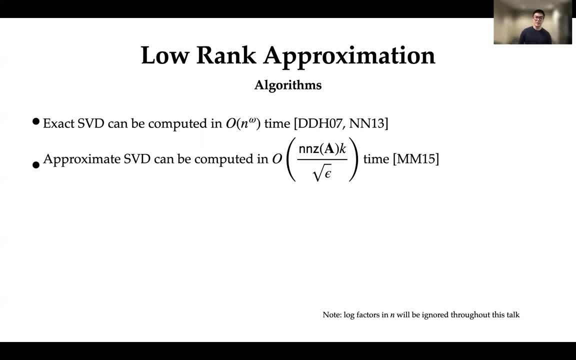 square epsilon time, And here NNZ of A refers to the number of non-zero entries of A, and epsilon is an accuracy parameter, And here the notion of approximation is that we want to output a matrix, A hat, such that A minus A hat in the spectral norm is equal to A minus. 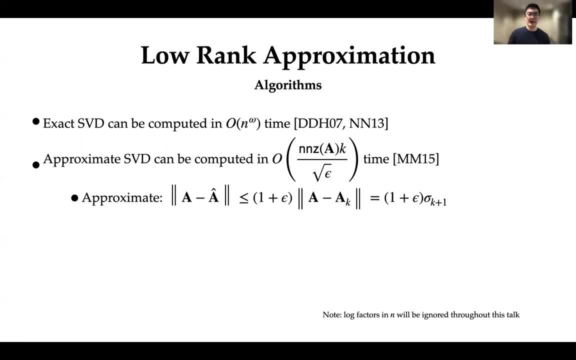 A k in the spectral norm, which is at most 1 plus epsilon times A minus A k in the spectral norm, which is also the same thing as 1 plus epsilon times sigma k plus 1.. So what this means is that A hat will remove all the top singular values of A, except for those that 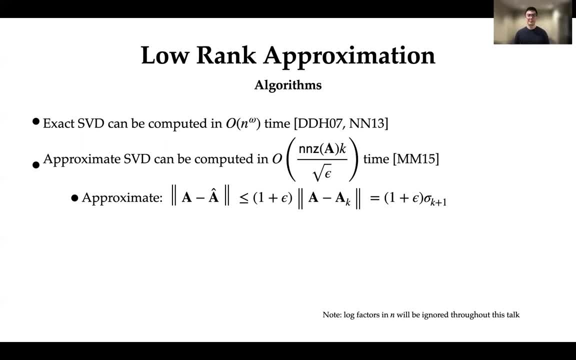 are at most a 1 plus epsilon factor larger than sigma k plus 1.. Now this NNZ of A times k over square epsilon time has been a long-standing barrier and a natural question that we could ask is: can we compute the NNZ of A times k over square? 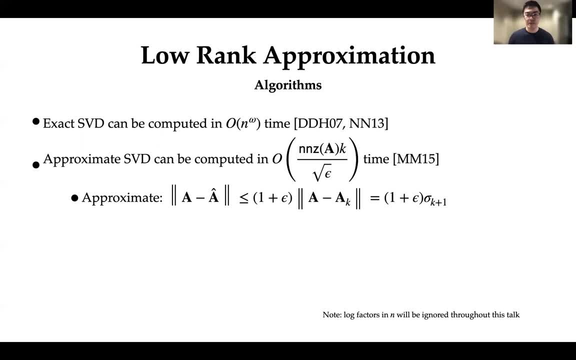 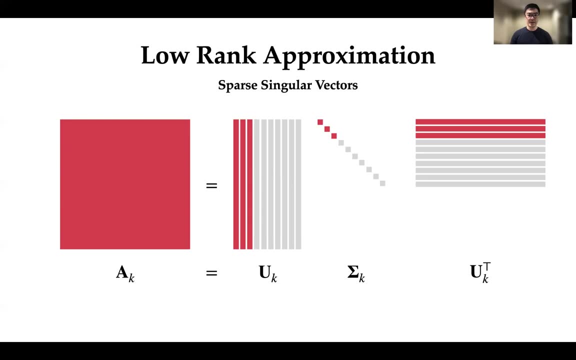 epsilon time. Can we get an algorithm that's faster than this, if we assume that the top k singular vectors are sparse? So what do we mean by sparse? So what I mean is that if I look at A, k, the optimal rank, k approximation given by the SVD, then the top k vectors will be: 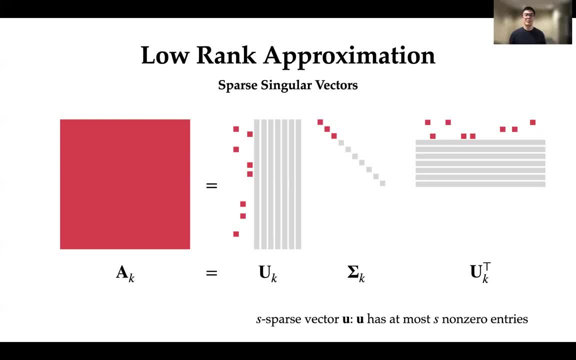 s-sparse, meaning that these top k singular vectors only have at most s non-zero entries each. Now, our main theorem in this setting is that the top k singular vectors are sparse. So what we're going to do is we're going to compute the NNZ of A times k over square epsilon times. 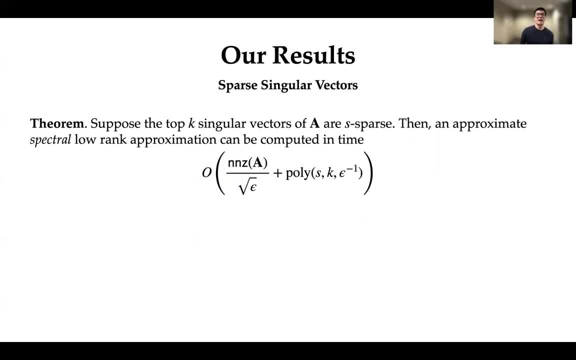 k порядuring a term, these tensors. So if I look at the dominant theorems, which is NNZ of A over square epsilon, this means that if the top k singular vectors are sparse, then we can see a factor that is at the maximum. 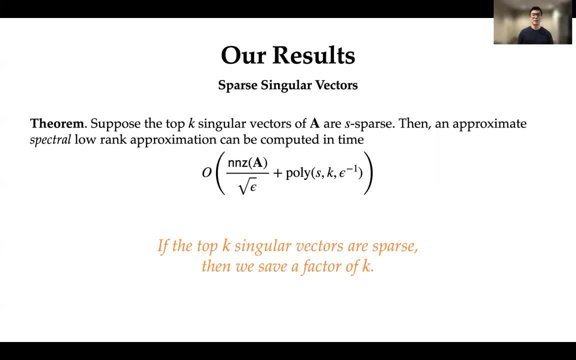 vector. That's a typical expectation to say that if I compute n nz of a times k number of k over the best known spectral long approximation algorithm. Now, this is the result that I want to prove, but before I do that, I want to introduce some of our other results in the 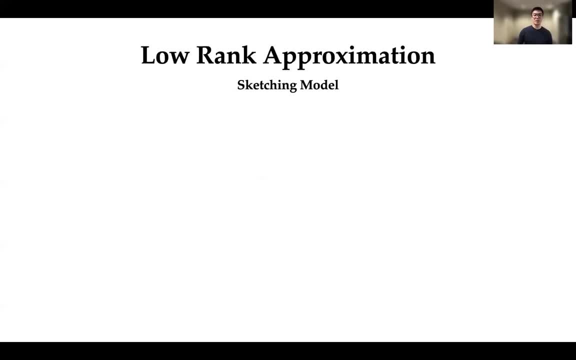 sketching model. So in order to do that, let me briefly introduce the sketching model. So in this model our input matrix A is observed through t linear measurements, and by that here's what I mean. So we first get to choose query matrices S, i, which is an n, by n matrix. 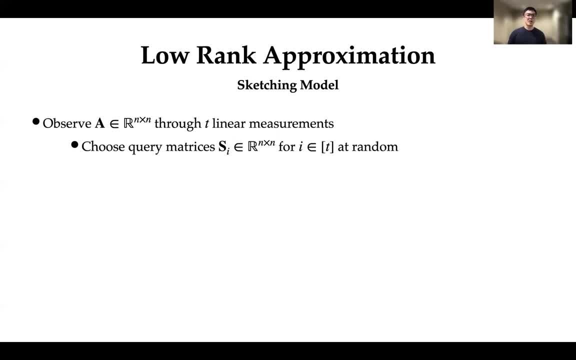 for i from 1 to t, and these query matrices can be chosen to be random. And then, after I choose these query matrices, I'll be able to observe the inner product between S, i and A, from i equals 1 to t. And finally, after I observe these linear measurements, 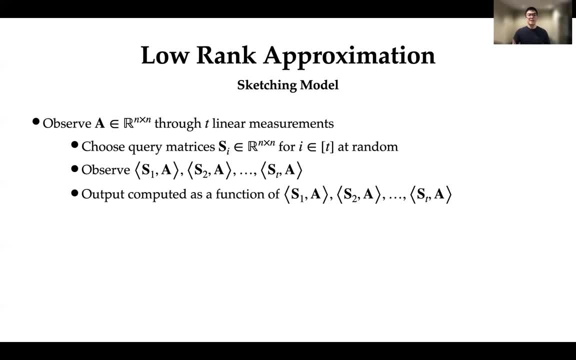 I can output. I compute my output as a function of these queries that I, that I observe. And here the complexity measure that we're trying to optimize is the number of measurements t. Now, in this model a Lorentz approximation has been studied in the past in the Frobenius norm. 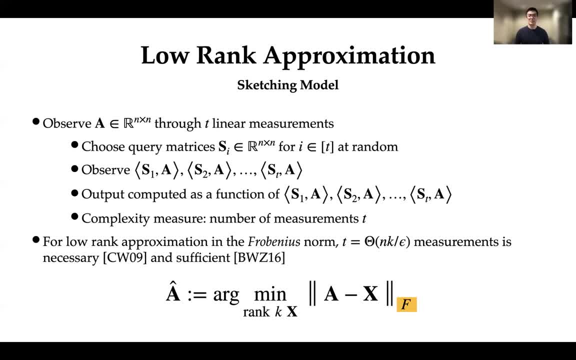 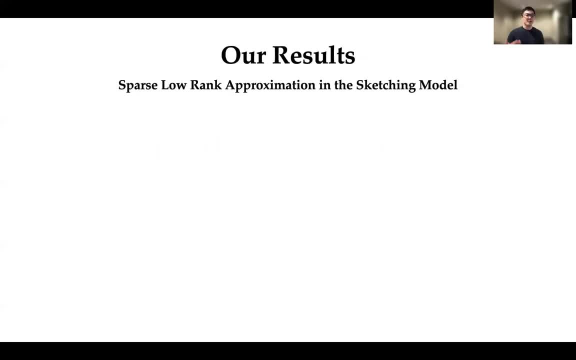 and it's known that nk over epsilon measurements is necessary and sufficient for this problem. Now again, we could ask whether sparsity could improve the situation. And this time we're going to be using sparsity in a slightly different way, where, instead of assuming that A has some natural sparsity attached to it, 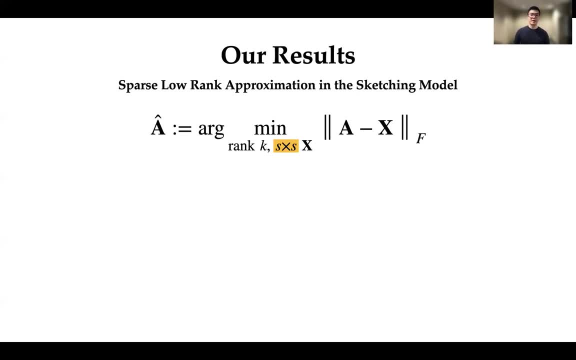 we instead change the optimization problem so that we explicitly search for an S by S matrix that approximates A. So, more formally, we want to find an A hat that minimizes A minus x, where x ranges over rank k matrices that are supported on an S by S sum matrix. 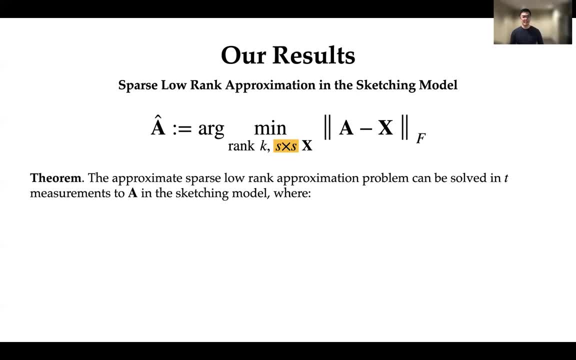 Now in this setting we show a variety of results and trade-offs where we can solve this problem: in t measurements where t can be taken to be sk over epsilon squared if we allow for the use of an exponential time algorithm but we get to output a genuinely S by S matrix k hat. Now this exponential time might be. 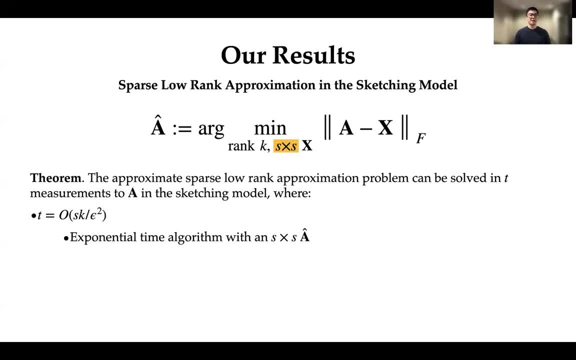 undesirable, but we still get a very small measurement complexity of sk over epsilon squared. So note that this actually doesn't depend on n in a polynomial way. Now this exponential time is undesirable. so our second result is that if we allow for a slightly increased number of measurements, so if we use s squared, 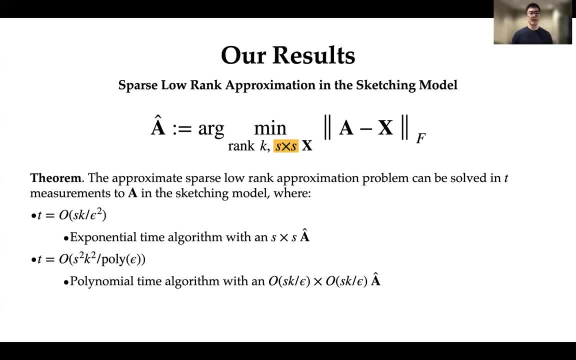 times k squared over poly epsilon, then we're actually able to get a polynomial time algorithm, with additional caveat that we output a relaxed sparsity. So our output matrix is sk over epsilon times sk over epsilon. And finally, we can actually obtain a further improved measurement complexity. 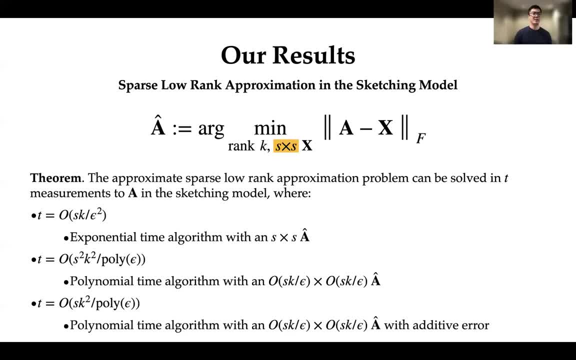 with polynomial time if we allow for an additive error instead of the earlier relative error notion that I mentioned. So this is all I want to mention for now for these results, and I'll refer you to our full version of our paper for additional details. So the rest of this talk I'll be coming back to this result on computing a spectral low-end. 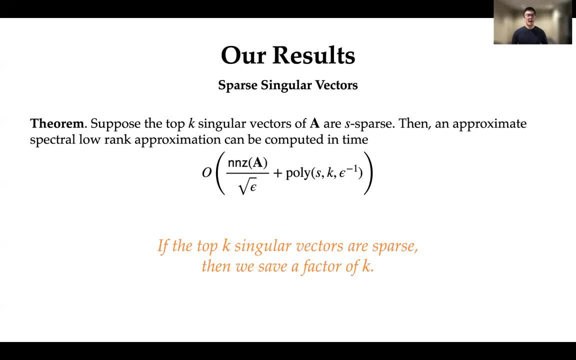 approximation in an Nz of A over square root of x. So I hope you enjoyed this talk and I'll see you in the next one, Thank you. So, as an overview of how we take this approach, I'll first reduce our tasks to finding the support of the singular vectors. 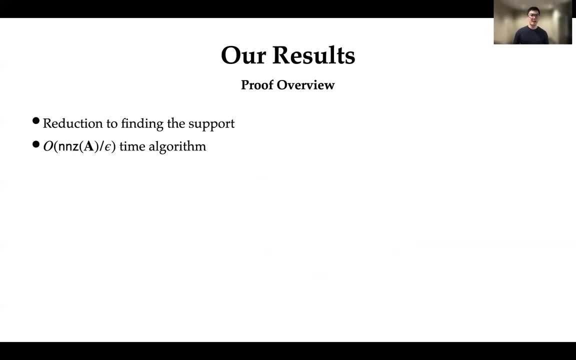 and once I do that, I'll show you an Nz of A over epsilon time algorithm for this reduced task of finding the support, and then I'll show you how to improve this to Nz of A over square root epsilon. Now, one thing to note is that this: 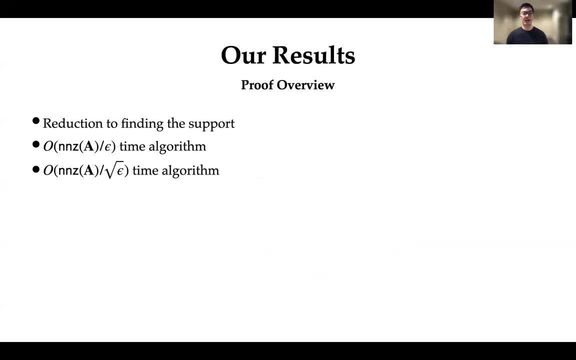 improvement from the dependence of epsilon to square root. epsilon is kind of standard in previous works, but in our work it's actually a very nontradial part of our algorithm, So it's not just a classical use of acceleration using captured polynomials. Without further ado, I'll get into this first step, which is the reduction to finding the support of. 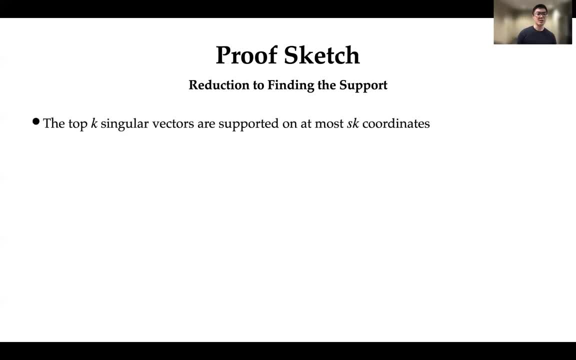 the singular vectors. So the first thing to note here is that the top k singular vectors are all actually being a question mark to the real method of simpleSimpler, so breaking them down and supported on a set of, at most s times, k coordinates, where I have s coordinates for each of the 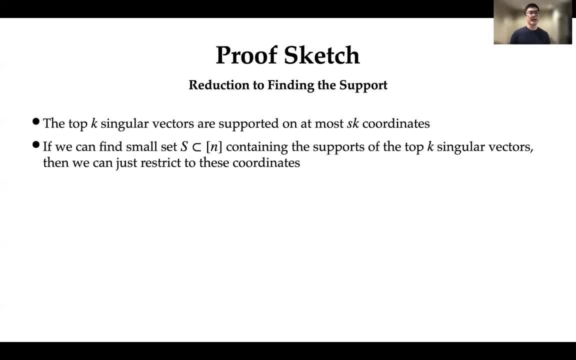 k sparse singular vectors. Now the claim is that if we can then find a small set of s that contains the support of these top k singular vectors, then what we can do is we can just restrict to these coordinates and then solve lower approximation on this submatrix. on. 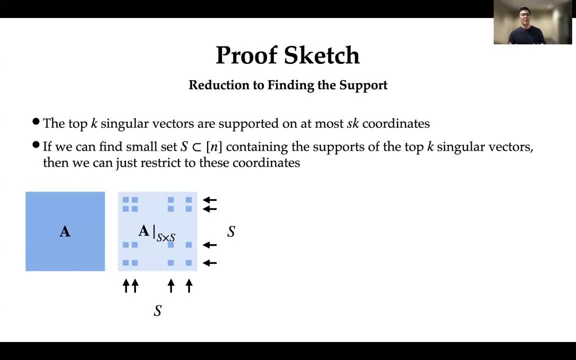 this restriction. Now to briefly see why this is the case. so consider this a bar s by s, which denotes the restriction of the submatrix, And what you'll notice is that if I consider the top k singular vectors ui, then a times ui in the two norm is exactly preserved by. 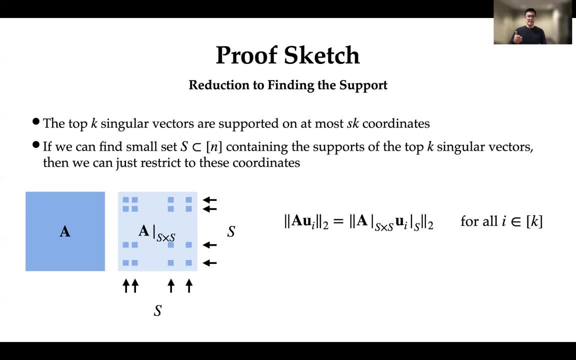 restricting to the submatrix, And this is basically because ui is just zero anyway, outside of the support. However, if I consider the top k singular vectors, then ui is exactly preserved by restricting to the submatrix. So if I consider any other vector, then what happens is that the value 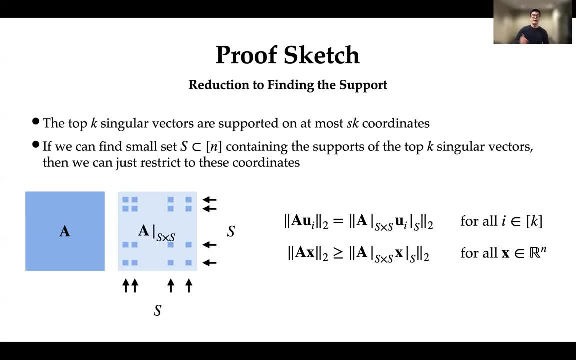 of Ax in the two norm can only decrease, since I'm just throwing away mass. So what this means is that the top k singular vectors are preserved under this restriction, while the rest of the singular components can only decrease. So that's the intuition for why it reduces. 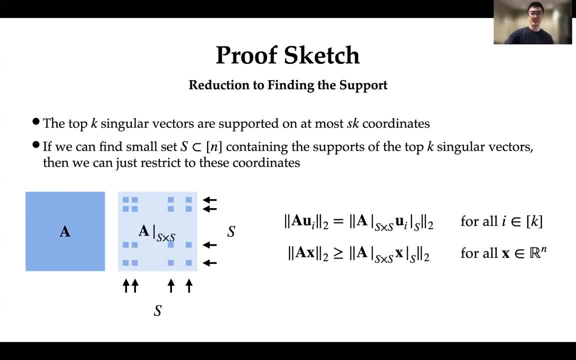 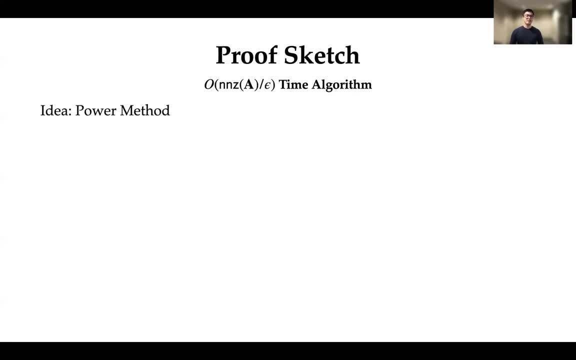 to finding the support of the singular vectors. Now I'll move on to the NNC of AO-Repsontine algorithm. So the main idea for this step is to just use power method. So the first thing I'm going to do is I'm going to go ahead and show you the pseudocode. So the first thing I do is: 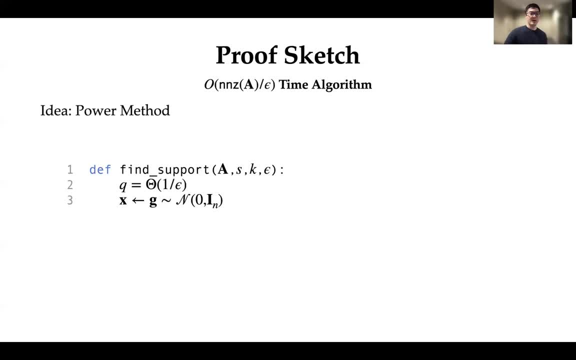 I'll set a parameter q equal to 1 over epsilon and I'll initialize a vector x, which is going to be my iterate, by a single Gaussian vector, g in n dimensions. And then, for q iterations, what I'll do is I'll repeatedly set x equal to a times x. 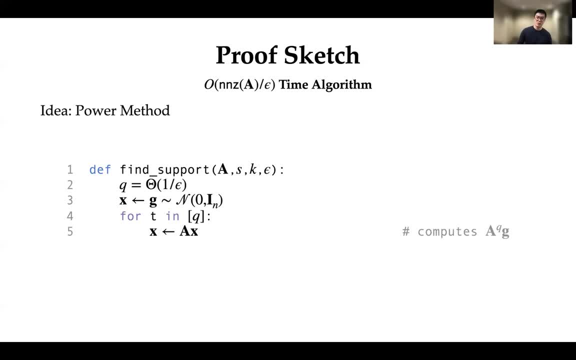 So this essentially accumulates the product a to the q times g, And note that each one of these matrix vector multiplications takes time NNC of a, and I'm doing this for 1 over epsilon iterations, which gives me the running time. And then, finally, what I'll do is I'll 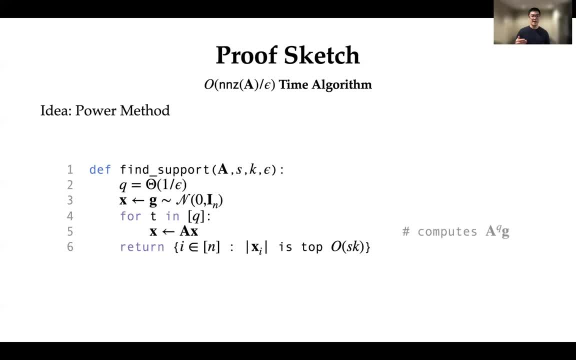 put the coordinates that correspond to the O, largest coordinates of x and absolute value. Now this is the algorithm, and let's see why this works. So first I'm going to think about a to the power of q, And the first thing I'll do is: 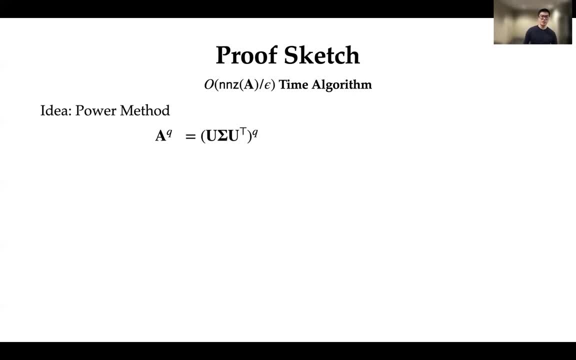 I'll write this and it's SVD. So this is the same thing as U sigma, U transpose to the power of q. And if I expand this matrix product out, you'll see that the U and the U transpose cancel out because the U has orthonormal columns. So this will give me U times sigma. 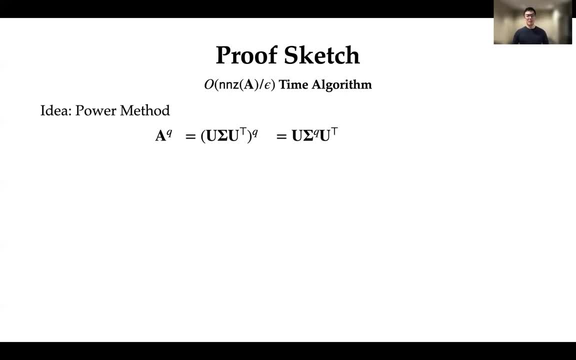 to the power of q times U transpose. Now let's think about what the sigma to the power of q does to the singular values. So suppose that I have singular values, let's say three of them, that are each separated by a factor of 1 plus epsilon, And this is the singular values of a. Now what happens? 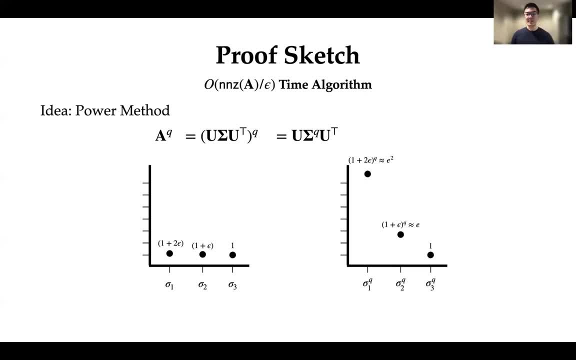 when I take the qth power of these singular values is that each of these 1 plus epsilon factor gaps are then boosted to constant factor gaps. So what this means is that, for example, if I have any singular value that's a 1 plus epsilon factor greater than 1 plus epsilon, 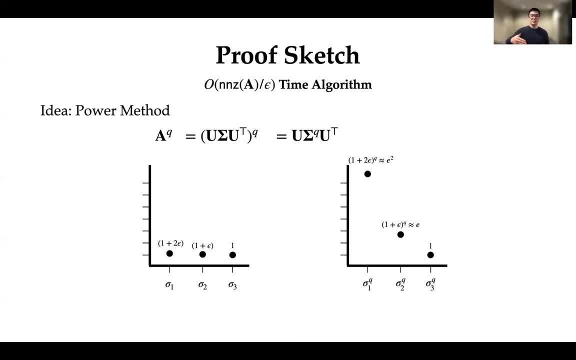 factor greater than sigma k plus 1, then these are all going to be a constant factor larger in the matrix product a to the q. So with that in mind, let's go ahead and see what happens. when I find a to the q times this Gaussian vector g. 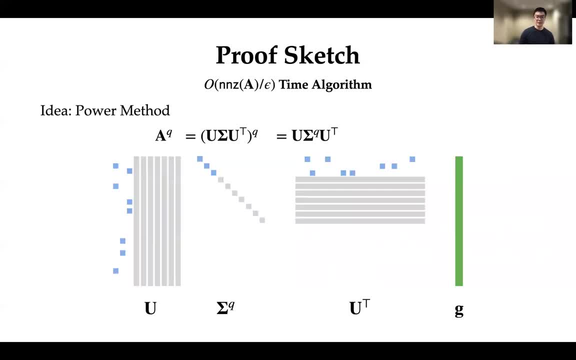 So first I'll write a to the q in terms of its SVD, like I did before, And let's first see what happens to this first matrix vector product. So here, notice that U transpose has orthonormal rows. So what this means is that if I multiply this matrix by a Gaussian, 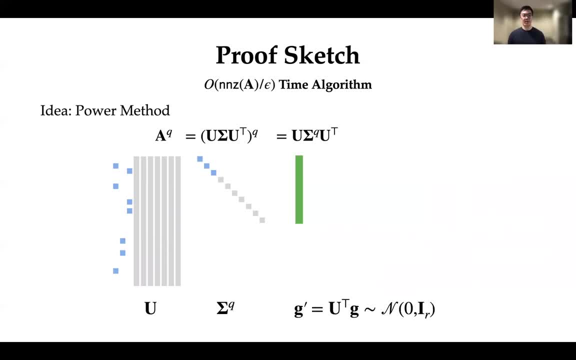 vector g, then what I'm going to get back is another Gaussian vector, a vector that's distributed as a Gaussian, that's only in r dimensions, where r is the rank of the matrix. And then next I'll multiply this Gaussian vector by this diagonal matrix sigma to the. 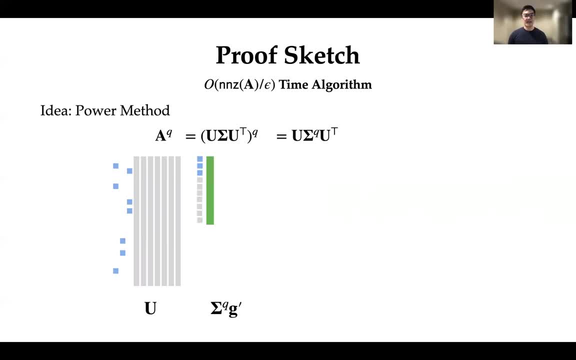 power of q, And what this gives me is a different Gaussian vector where each of the two matrix coordinates is scaled by sigma i to the power of q. And since these Gaussian entries are basically just like sine flips, they don't really affect the order of magnitude of these. 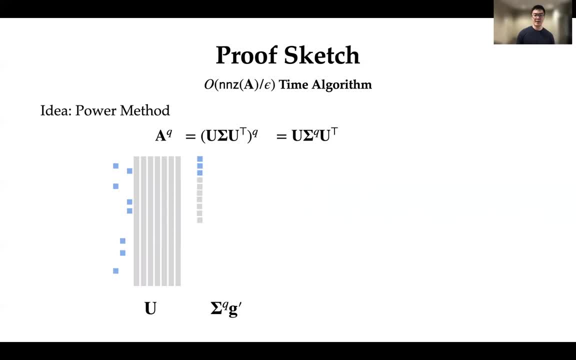 entries. I'm just going to throw this away for simplicity. And then, finally, I'm going to look at this matrix vector product, And what this does is it essentially gives you a linear combination of the singular vectors of a, where the i-th singular vector, which 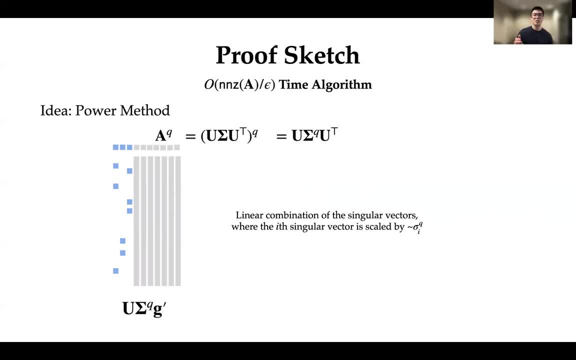 is a vector, is scaled by a coefficient that's roughly on the order of sigma i to the power of q. And again recall that any singular value that's larger than the factor of 1 plus epsilon, than sigma k plus 1, is actually scaled a constant factor larger than anything below. 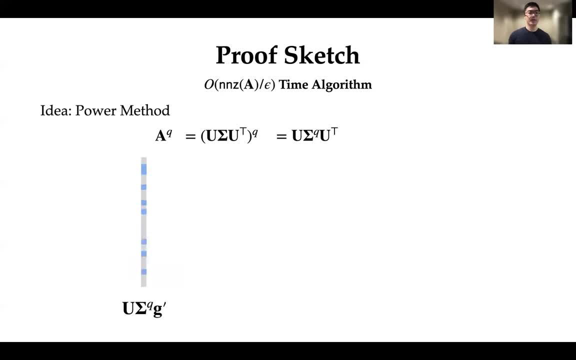 sigma k plus 1.. So, as a result, all I get back is this vector where I'll see all these coordinates that correspond to the top k singular vectors. So what this means is that I can just read off of these top sk coordinates that are the 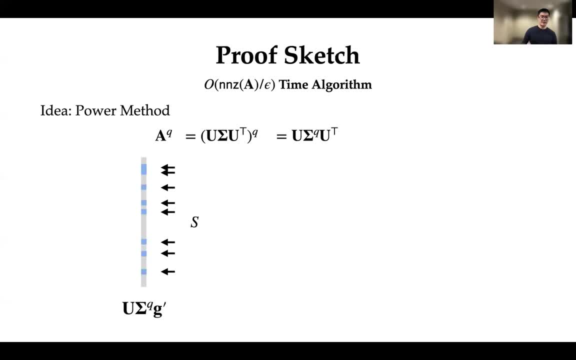 largest in this resulting vector and this will give me my support superset S that I want. And that concludes the nnz of a over epsilon time algorithm. Now, in order to boost this to an nnz of a over square root epsilon time algorithm, the initial thought might: 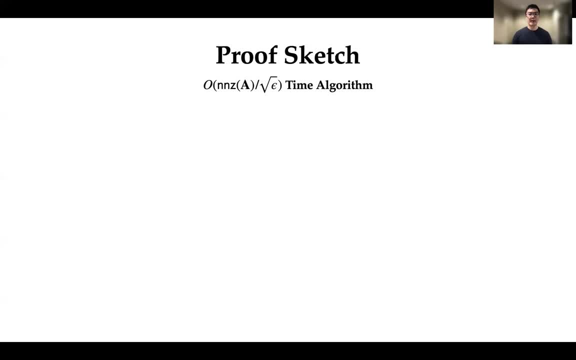 be to just use Chebyshev polynomials. So let me go over what this idea is and why it doesn't work. So the idea for using Chebyshev polynomials is that I want to replace the use of a to the power of q with t to the a where t is some degree square root, q polynomial instead. 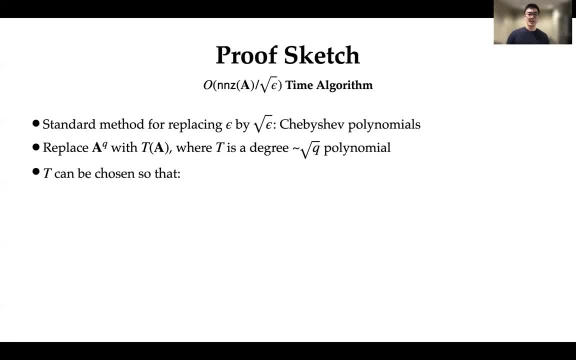 of a degree q polynomial. So the idea is to choose t, so that t of x is at most 1, and so whenever x is an entry, that's at most the k plus 1 singular value, and whenever x is at least 1 plus epsilon times the k plus 1 singular value, then I want the value of. 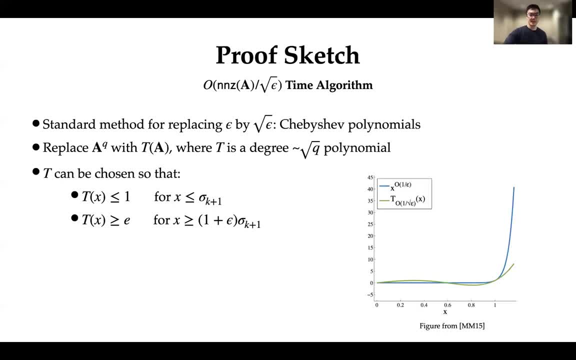 the polynomial to be at least a constant Now. so this looks something like this And this has worked in the past, for example for standard Lorentz approximation. But what's the problem here? The problem here is that t depends on sigma k plus 1.. 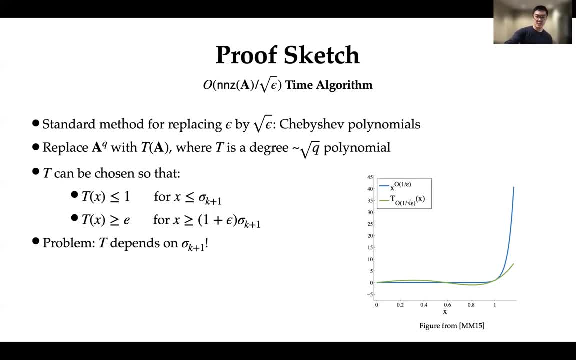 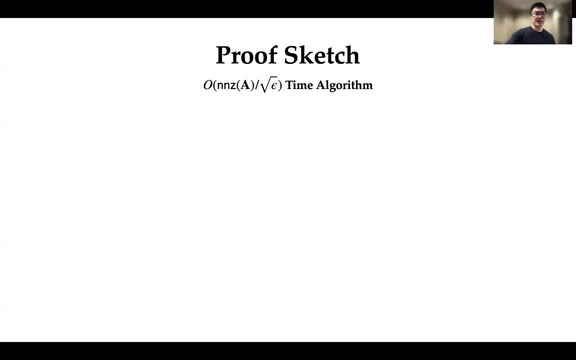 And we don't know the value of sigma k plus 1, which means that this approach cannot work, at least as is naively. So what's our fix? So the first thing we do is that we note that we can still run the previous algorithm if we set epsilon equal to square root epsilon. 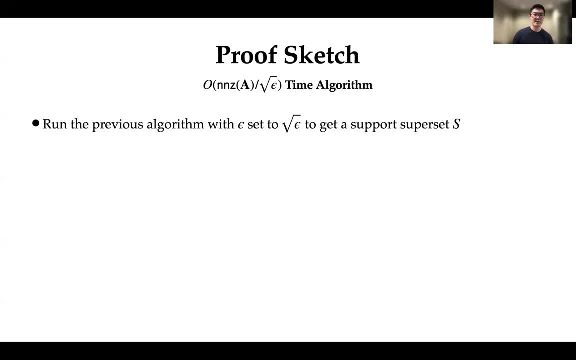 instead, And this will still get us some support superset S that gives us some sort of approximation. Then what we'll do is we'll use this support superset S to obtain a ring k approximation, a hat Of this submatrix restricted to S, And then next, then we'll show that we'll be able to. 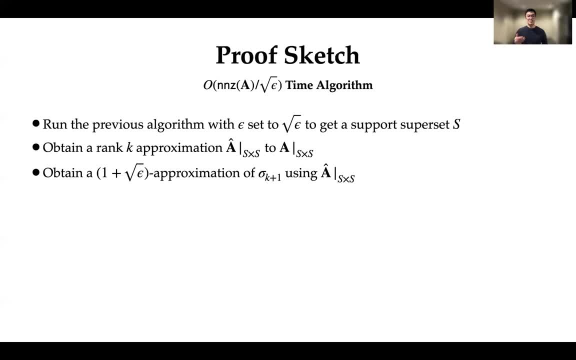 get a 1 plus square root epsilon approximation to sigma k plus 1 using this ring k approximation And then finally, once we have this 1 plus square root epsilon approximation to sigma k plus 1, then we can actually exactly get sigma k plus 1 up to a factor of 1 plus epsilon. 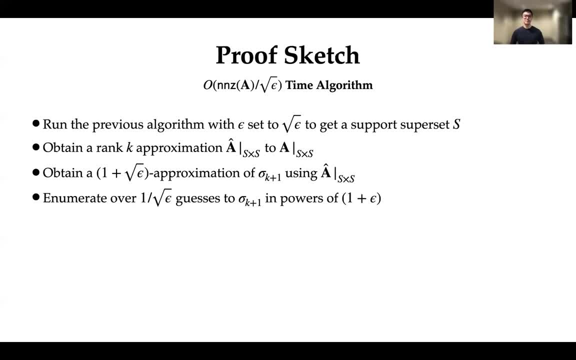 by making 1 over epsilon, 1 over square root epsilon guesses. So this is just by noticing that 1 plus epsilon to the power of 1 over square root epsilon is around 1 plus square root epsilon. Now the non-trivial step here is going to be the third step. So this is the step that. 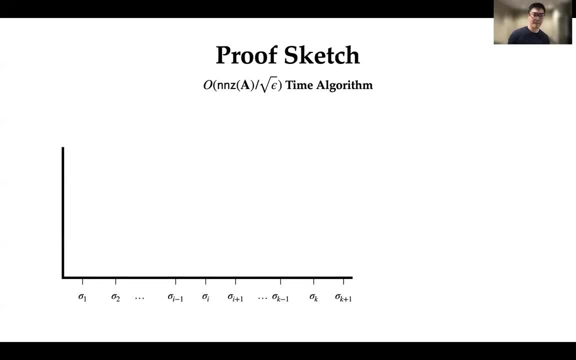 I'm going to go ahead and explain. So let's first plot the singular values of A as so, where I'm going to normalize the k plus 1 singular value to be 1.. And let's also plot The singular values of our submatrix A, restricted to S by S. And the first thing that you'll 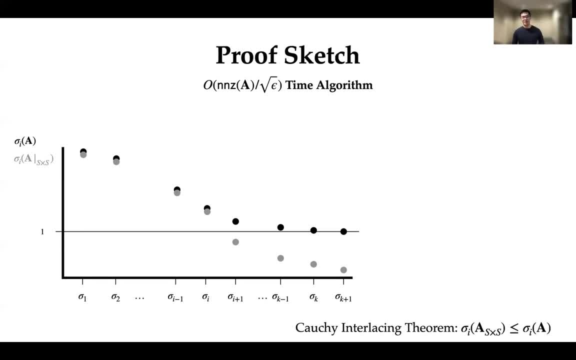 notice is that by the Cauchy interlacing theorem, the singular values of the submatrix is always at most of the singular values of the original matrix. And another thing that I want you to notice is that any singular value above 1 plus square. 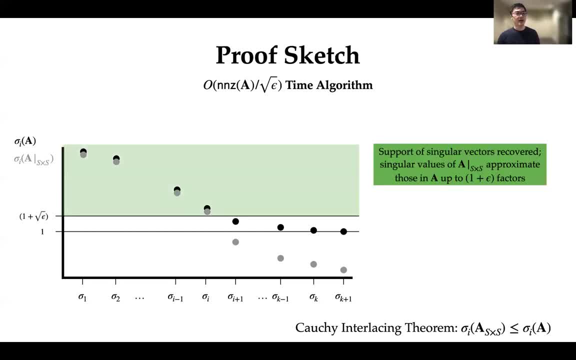 root epsilon is actually going to have a very good- they're going to be very good- estimates of the singular values of the Original matrix A, And this is because as long as the singular value is at least 1 plus square root epsilon, then we'll actually successfully recover the support of the singular vectors. 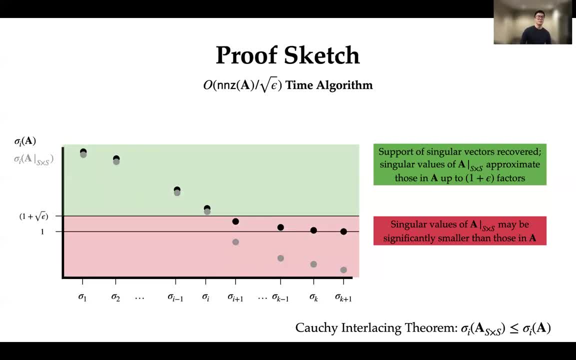 On the other hand, if we look at any singular value, that's at most 1 plus square root epsilon, then we may have a. it may happen that the singular values of the submatrix are significantly smaller than those of A. Now, in order to obtain our 1 plus square root epsilon approximation, 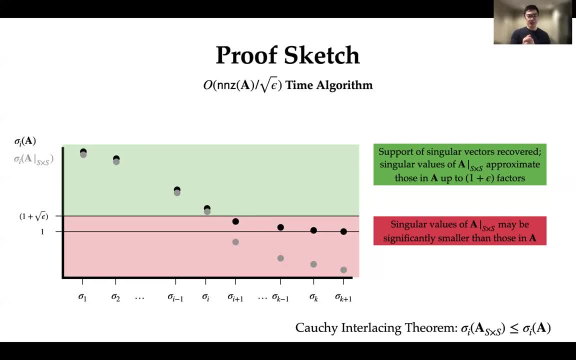 we basically want to find this index i, which is the largest index, such that the singular value sigma i is larger than 1 plus square root epsilon. So once we find this, we'll basically able to have like a reasonable estimate of sigma k plus 1 within a factor of 1 plus square root epsilon. 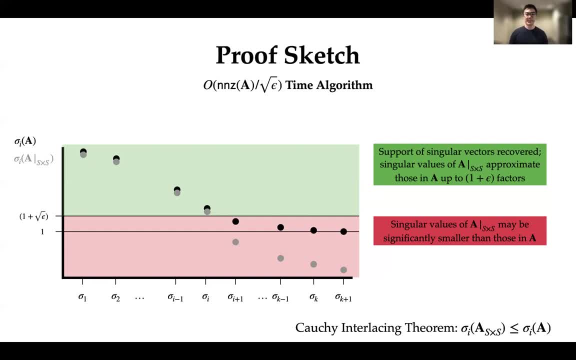 But the problem is we still don't know how to find this index, sigma i. So what's the idea for getting around this problem? So the idea is that we want to find singular value, Upper value, Lower value. So if we have a scalar matrix, we call this pointer from the lower down of the LNatched. 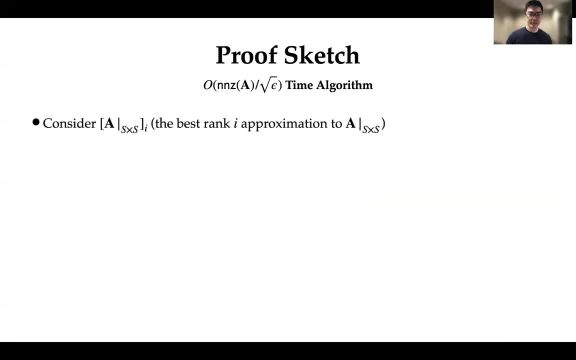 bottom, which is the prime of every value. So if we have a sum matrix of like of A'x, the sum matrix of A'x, we calculate the 어도 of the lower down of the Lnatched bottom And we calculate the value of the lower down of A'x, which is the prime of every value. 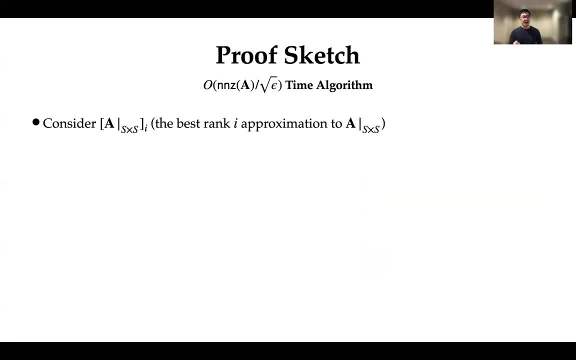 sigma i. So we have a lower-down value that approximately maps the lower bounds. So let's see what this means. So first consider the best rank i approximation to our sum matrix, A bar s by s. Then suppose that we calculate the operator norm of A minus this approximation. 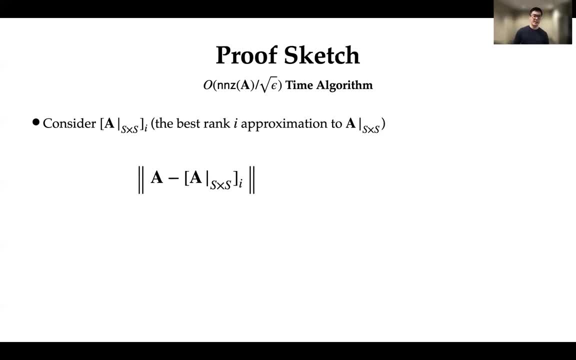 And know that this can be done in an entity of A over square root, epsilon time. since we're just computing singular values, a single singular value, Then this upper bounds, the quantity, the minimum over rink I. matrices X of A minus. 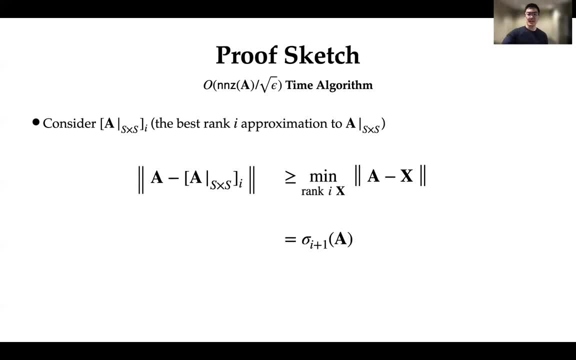 X in the spectral norm, But you'll notice that this is actually just the I plus 1 singular value of A. So what this means is that the spectral norm of A minus our rink I approximation to the submatrix serves as a valid upper bound on the singular values of A. 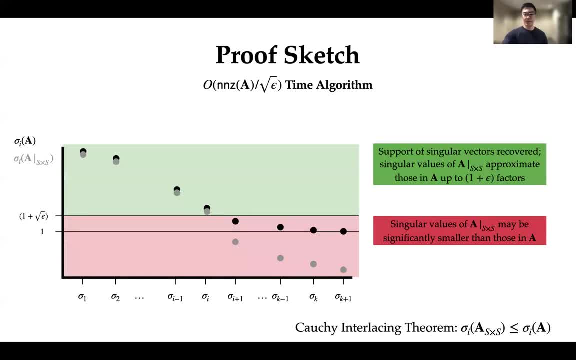 So, with this idea in hand, this leads to the following observation. So if we plot the values A minus the rink I minus 1 approximation of our submatrix in the operator norm, then these all give upper bounds on the singular values of A, while being: 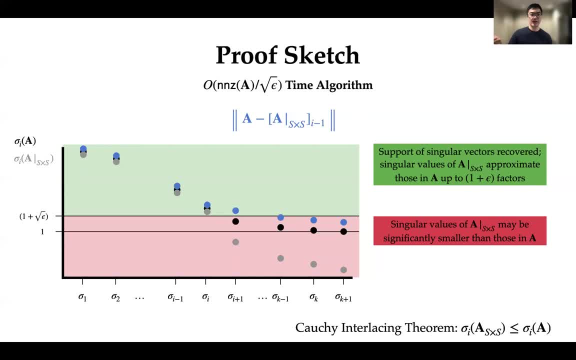 very close to these values, up to a factor of 1 plus epsilon, whenever the singular value is at least 1 plus square epsilon. So what we'll notice is that anything above this 1 plus square epsilon line, these upper bounds and lower bounds, will match. 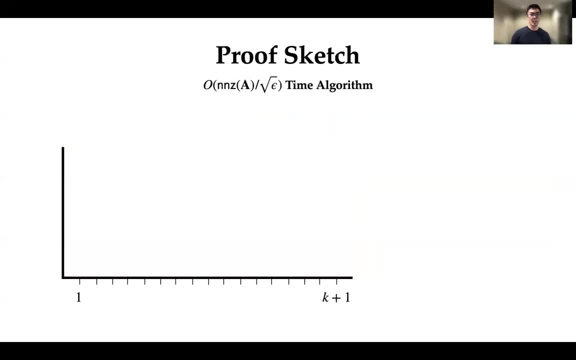 So this leads to the following algorithm. So what we're going to do is we're going to binary search for the smallest index, such that the smallest index i, such that the i-th singular value is the smallest singular value, that's at least 1 plus square epsilon. 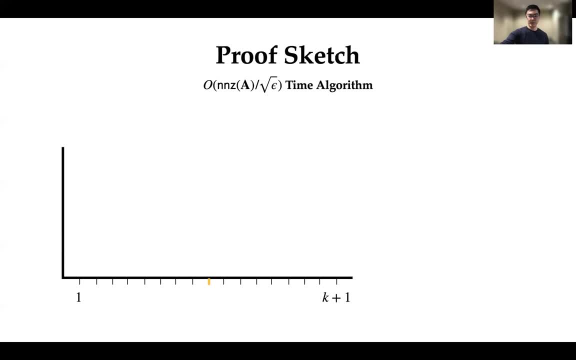 So let's say we start at index k over 2 and we compute the singular value upper bound as well as the lower bound using Cauchy interrelation theorem, and if we see that these two values are within 1 plus epsilon factors of each other, then we'll search for a lower index. 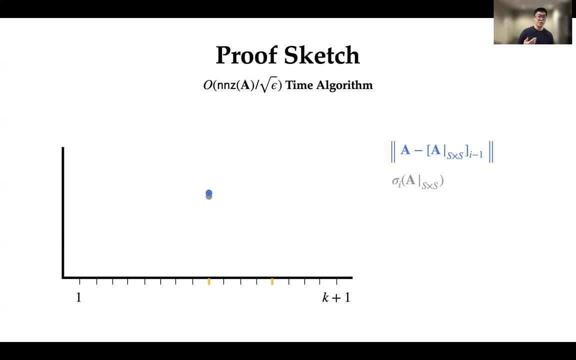 So let's say we look for the singular value corresponding to 3k over 4, and so we'll compute the upper bound and the lower bound, and this time, if we see that these two- upper bounds and lower bounds- are further than 1 plus epsilon, then we're going to search for a higher singular. 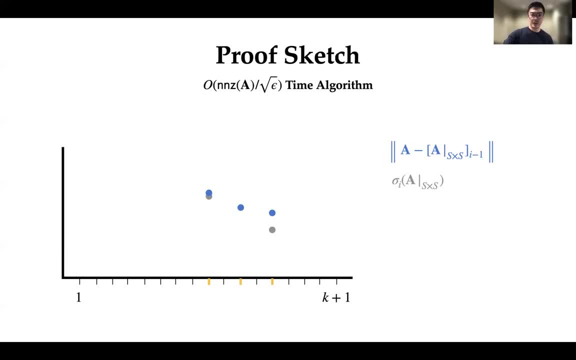 value. So let's say, we search here, We find the upper bound and the lower bound and if they don't match, we find the upper bound, lower bound for the next index and using this binary search algorithm we'll be able to find this index. i star, which is the uh, which is the smallest singular value, that's. 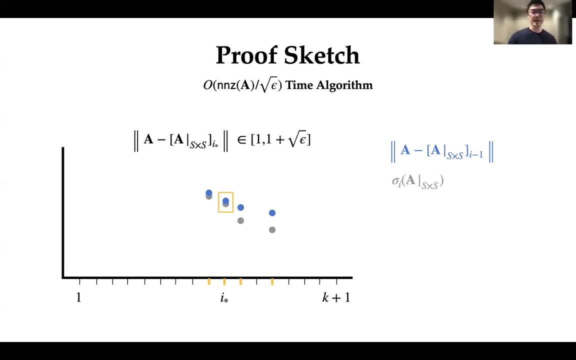 at least 1 plus square epsilon. Now, once we have this in hand, we can actually use the same trick as before to compute the singular value. that's right under this. So if I compute a minus, the i-th Rienke, i approximation Okay.